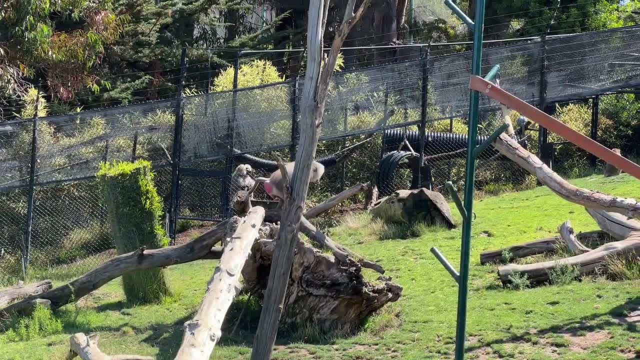 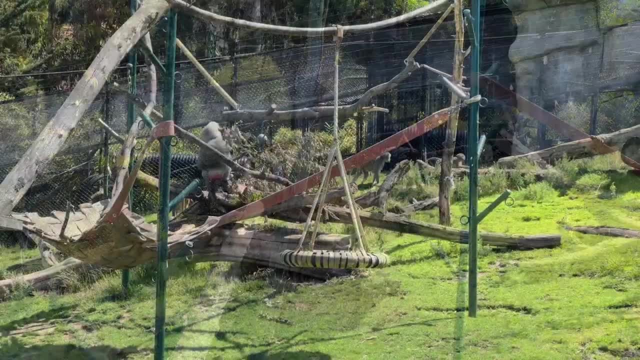 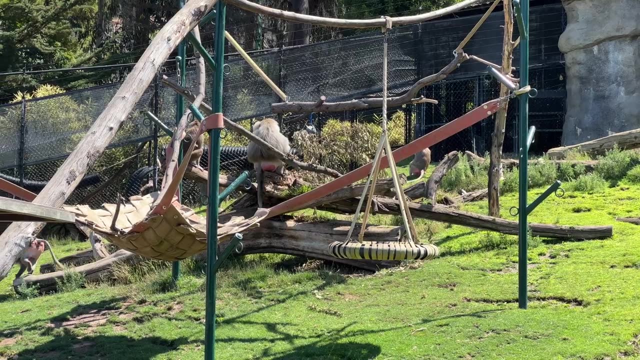 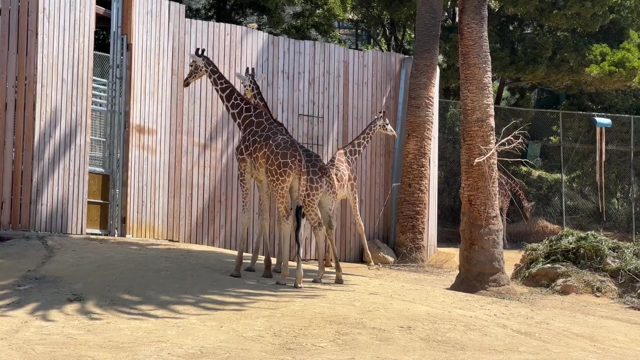 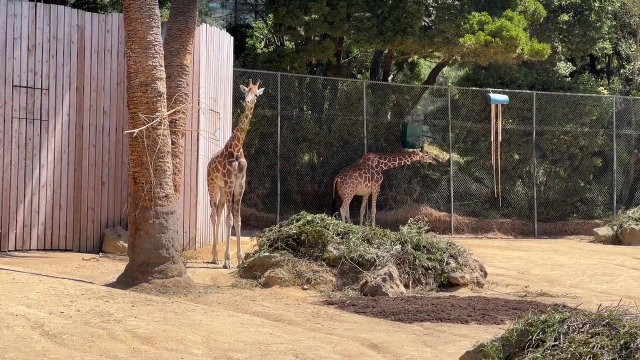 the baboon giraffe zebra. There is the great dry swarf. We are no longer in the wild. as we are starting our final day, I hope you have a wonderful evening. Enjoy the beautiful view of the beautiful and quiet tattooing. 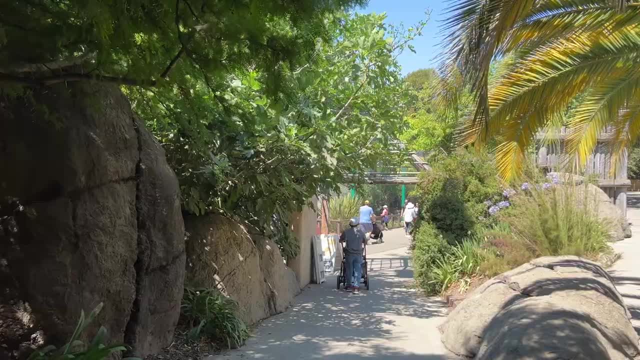 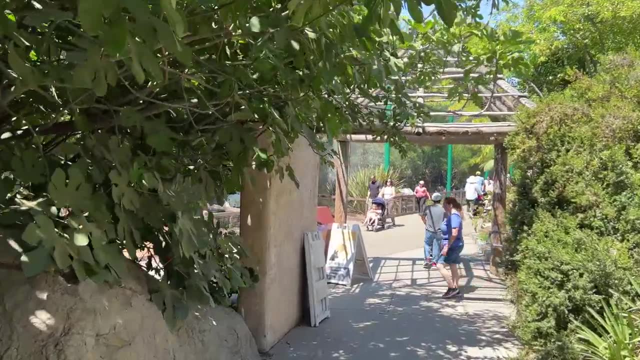 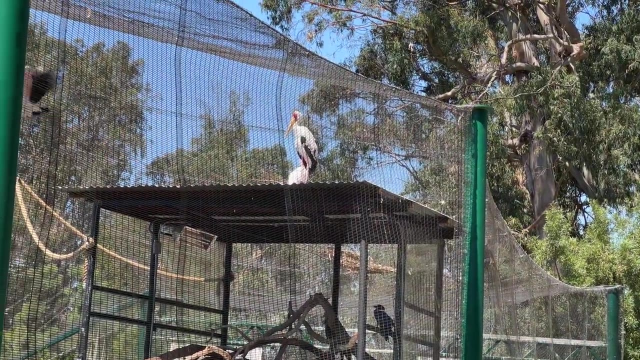 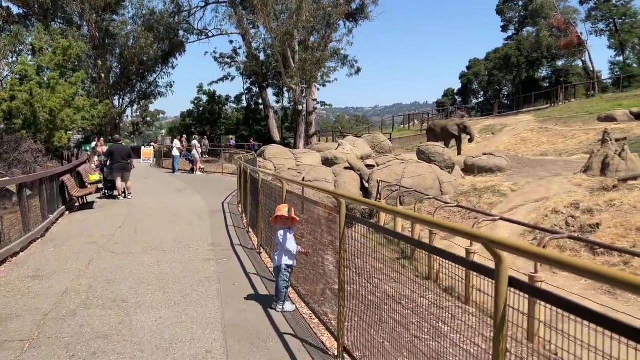 tree at the entrance. If you enjoyed this video, please like and subscribe to my channel. Thank you very much for watching. I am your host, Betsy Vitrano. Until next time, happy Celestino, my kid love the elephant. it's a huge elephant. look at him. it's looking at the elephant. 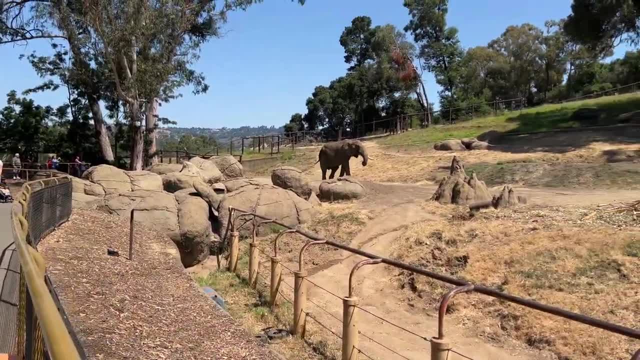 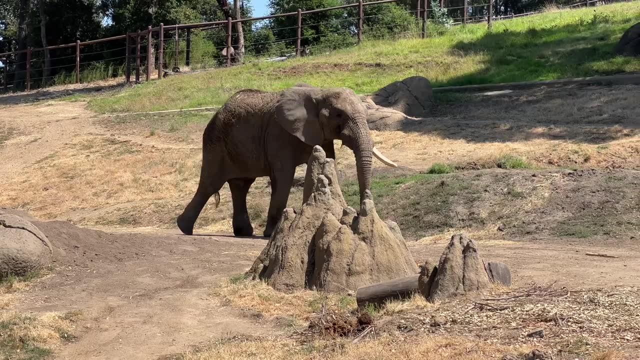 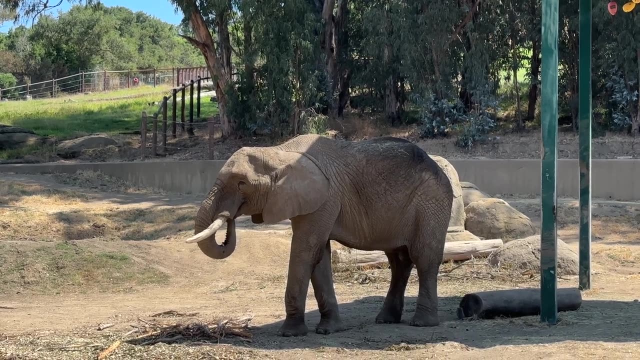 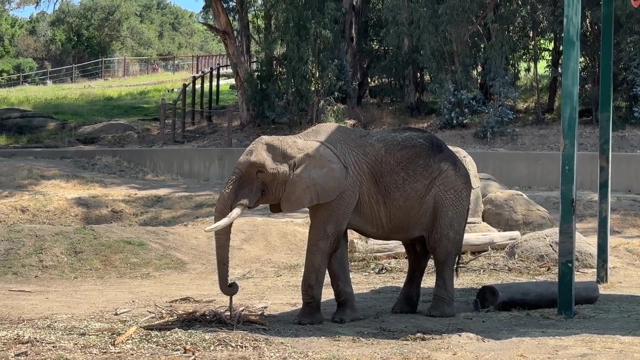 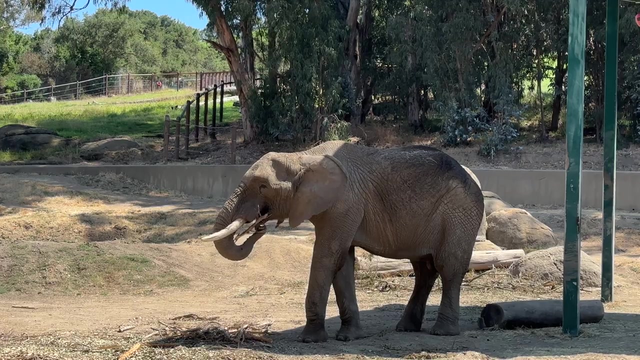 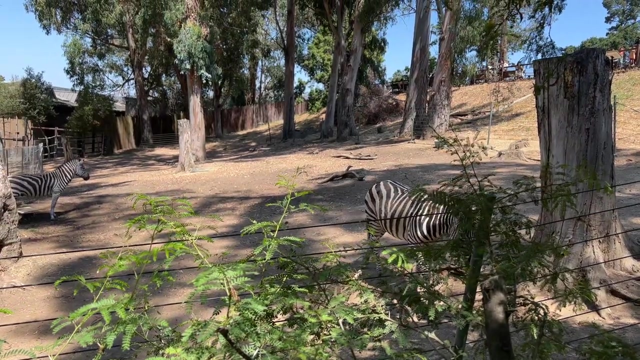 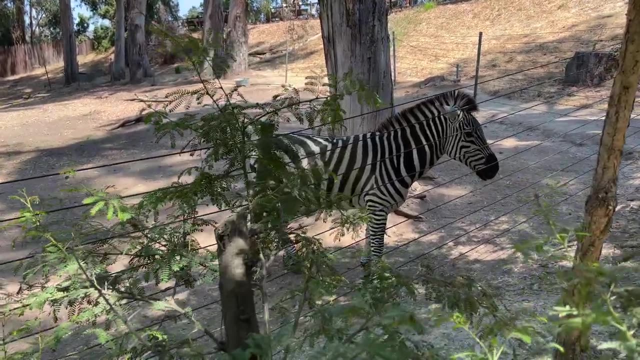 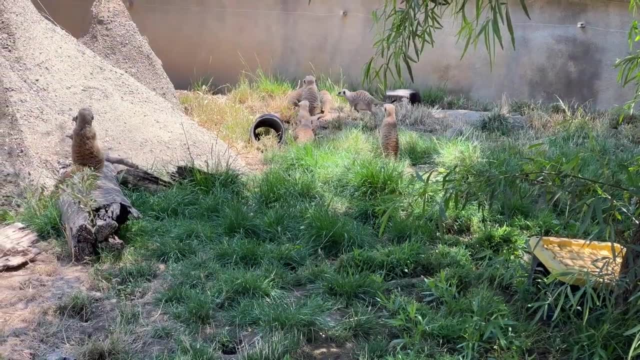 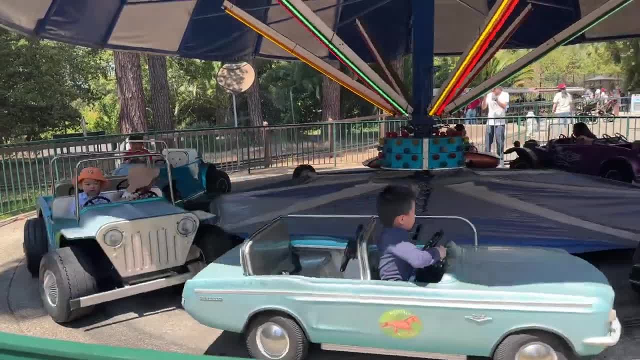 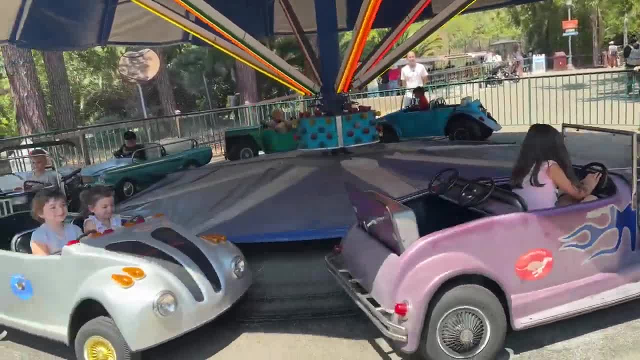 and this elephant is 25 years old and it lost one of the tusks. wow, we have a zebra. if you look at the all the animals here, they are pretty well fed and well taken care of. i would suggest you to take a detour to the right area. this is the place for the kids. the car ride is 2.50 cents per child. 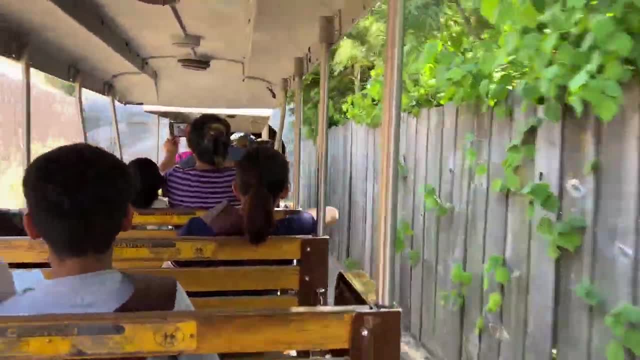 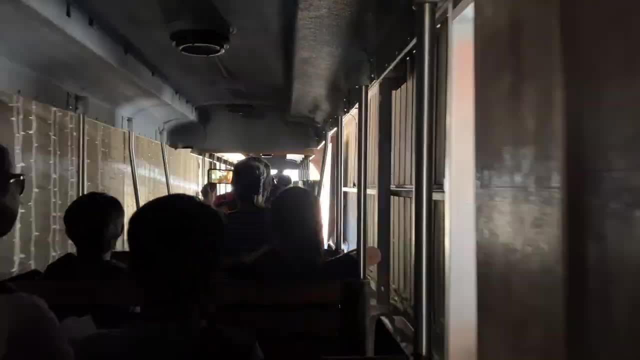 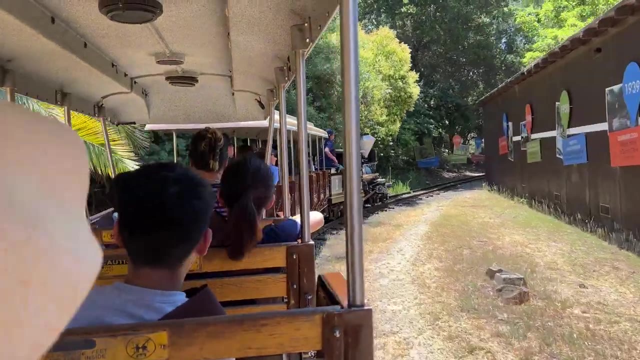 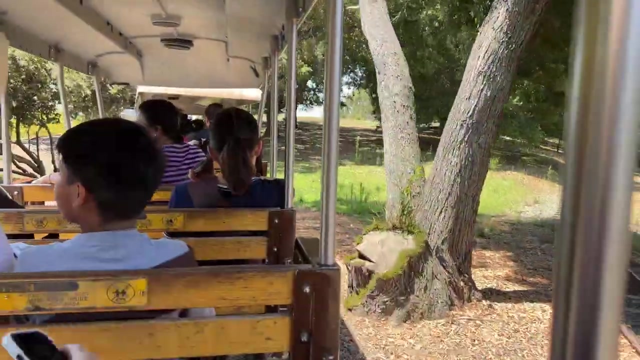 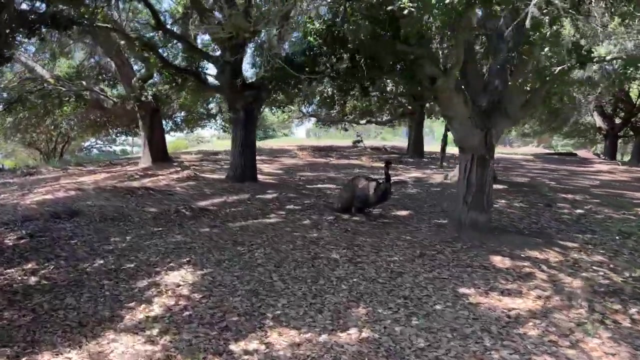 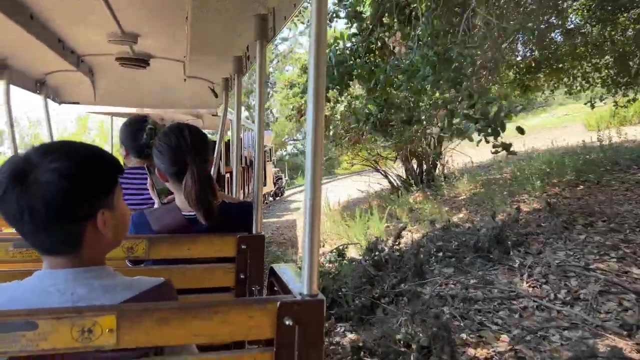 the train ride is five dollars per person and that train ride will take you to the wild australia region inside the park in which you can see the Aguadilla In kimotsu, Yukon кож hairs and the cat soup. the zoo is up in the hillside along the west side should open forили Mos Eis. the zoo is up in the hillside along the west side should open forily Mos Eis. not much people in the morning. any of the twisty months gone. the zoo is open in nine to ten minutes. not much people in the morning. any of the twisty months gone. the zoo is open in nine to ten minutes. 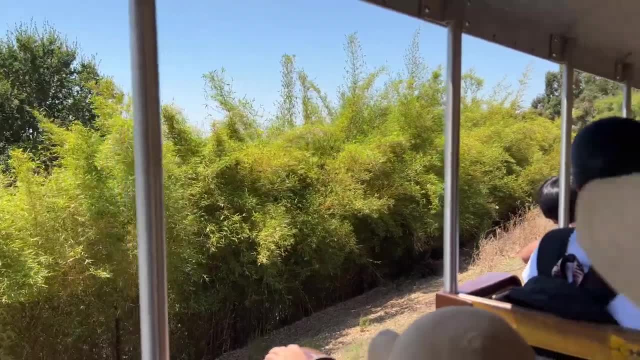 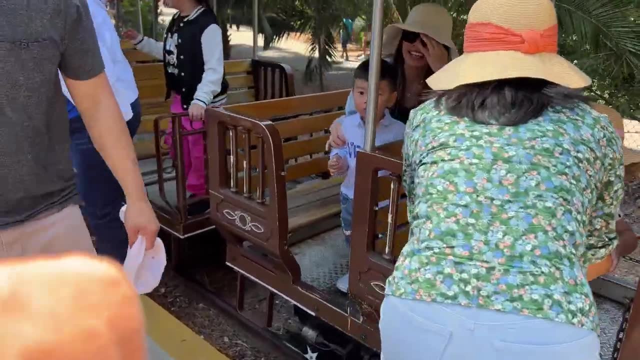 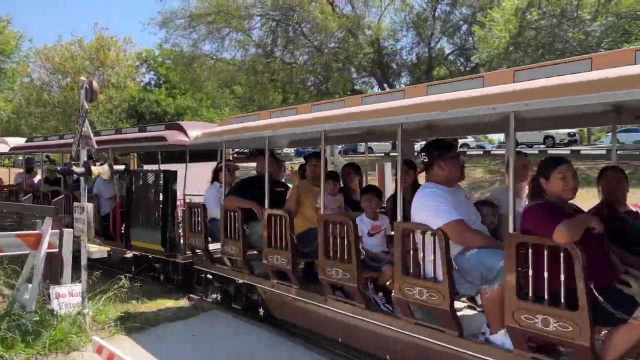 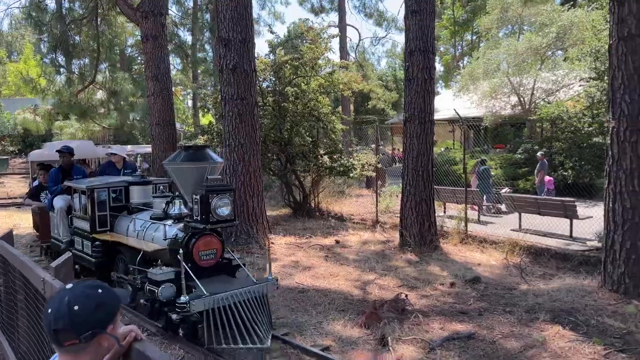 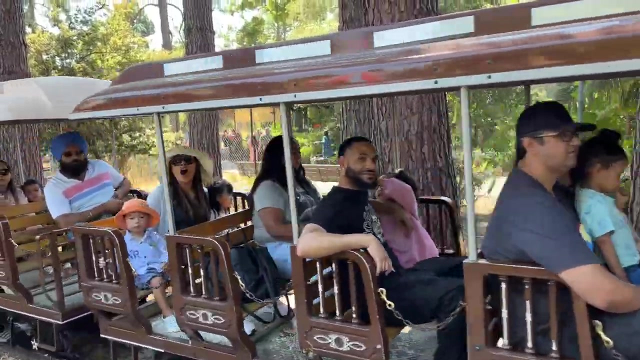 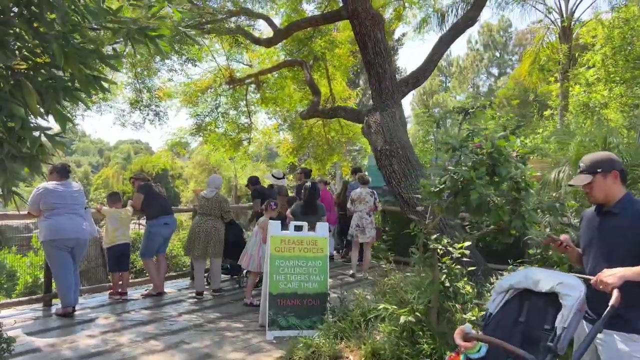 and the regeneration 20%. check out if you like it or not, 시면 Extra Dessert & Delicious information via many other places: rics&dstcom along the train ride. you can view the entire area below. After the train ride we get back to the Tiger area to take the Aerial tram or the gondola ride. 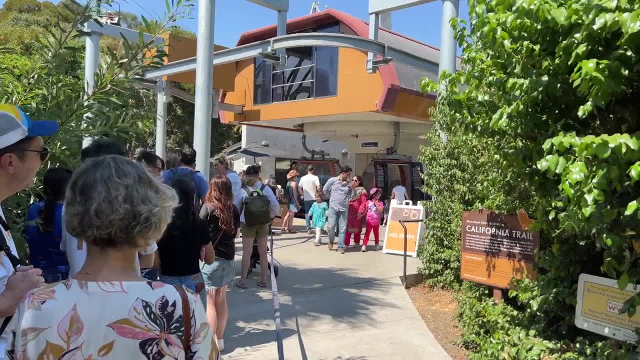 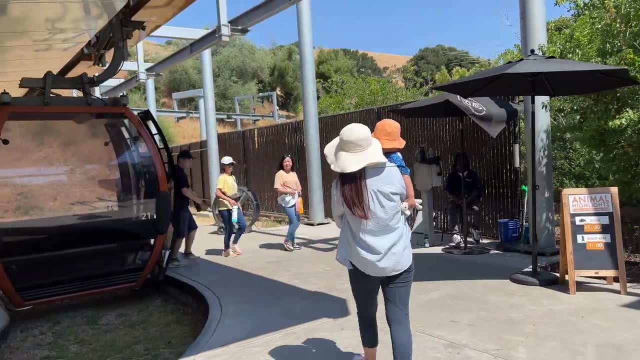 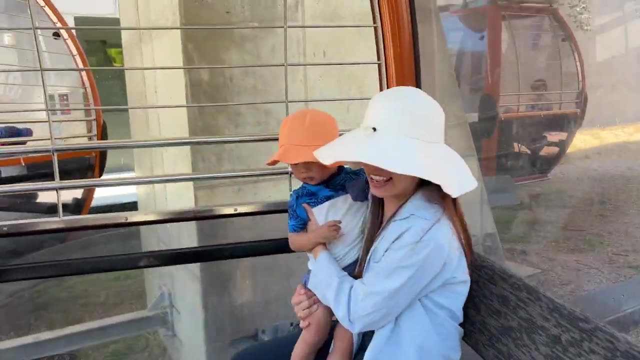 It takes about 5 to 10 minutes to get to the Tiger area. It takes about 10 minutes to wait in line for a ride to the Landing Cafe up in the California Trail region. The ride is free, so make sure you take it, because in the California Trail region you can see a lot of cool animals. 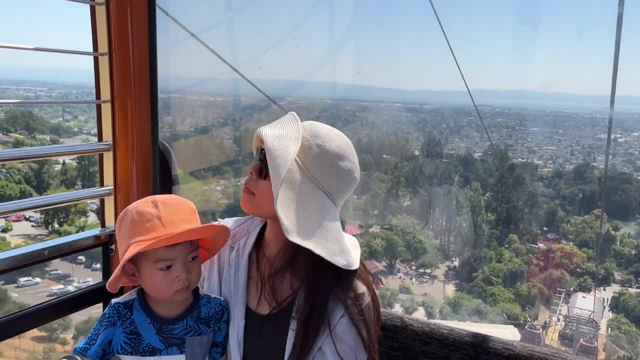 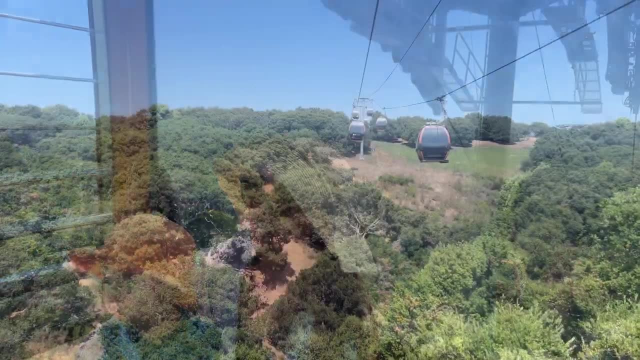 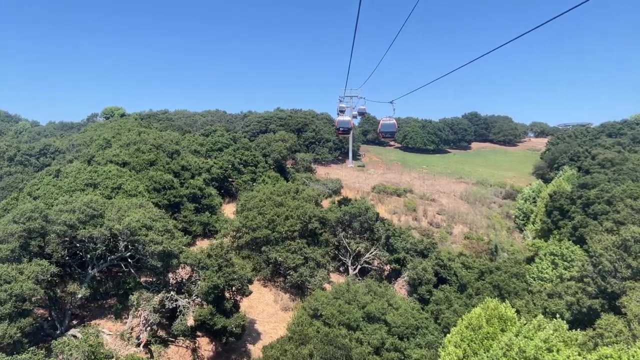 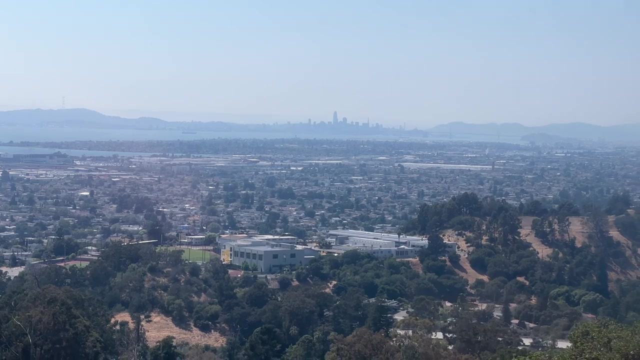 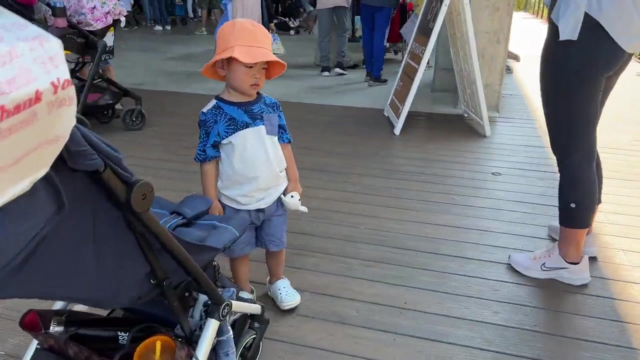 Cool Tom and his mom say hi to the people who go down. Rides are often not that tranquil, but the kids are super relaxed right after the ride. There are also no sad сделали, so they just ice eat. Sad stance: This is one of my favorite animal tracks in the nation because it has a Cross dicoté. but not all of man makes it still Absent-minded dude. This is a very arable Pat personakk ee. 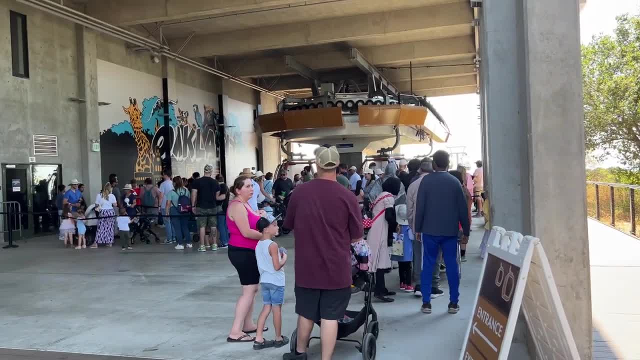 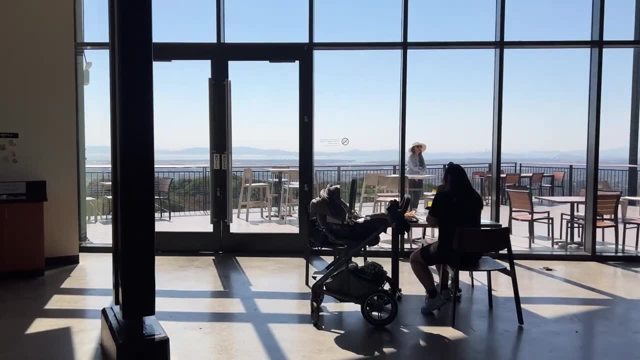 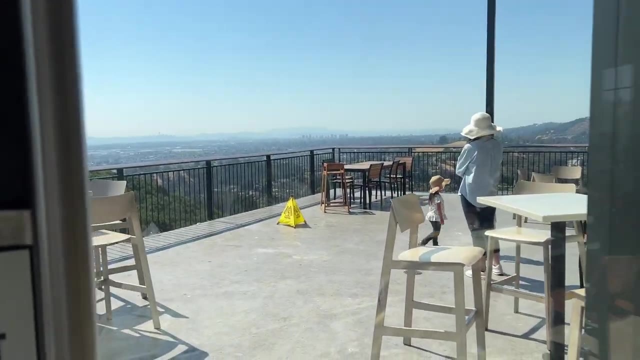 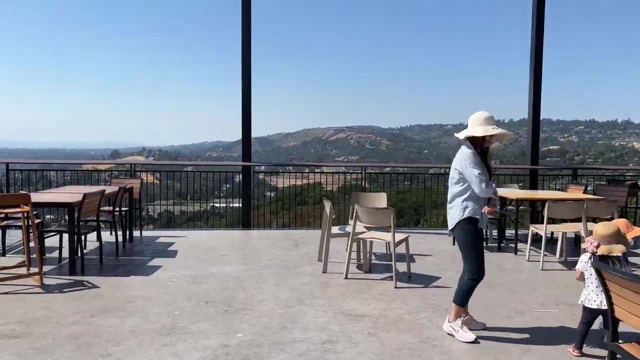 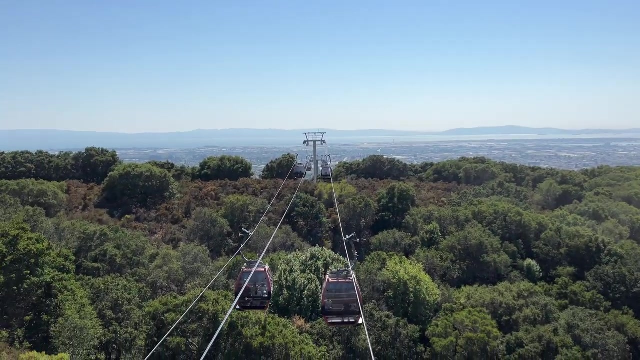 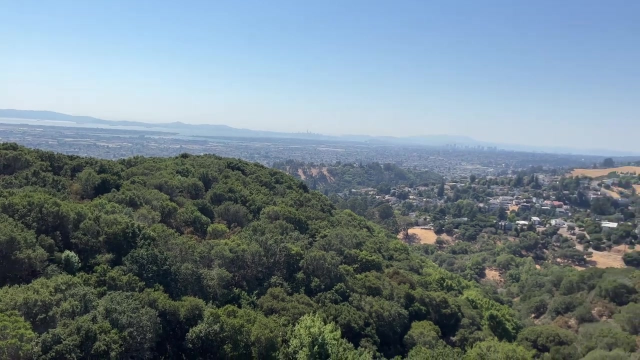 when we get to the landing cafe, we order some food. the food is pretty okay. however, the amazing thing about this cafe is the view. it is the five-star view. the food up there is, of course, as expensive as the five-star view: fries is $4.50, a cup of juice is $3.50, a burger is $17. 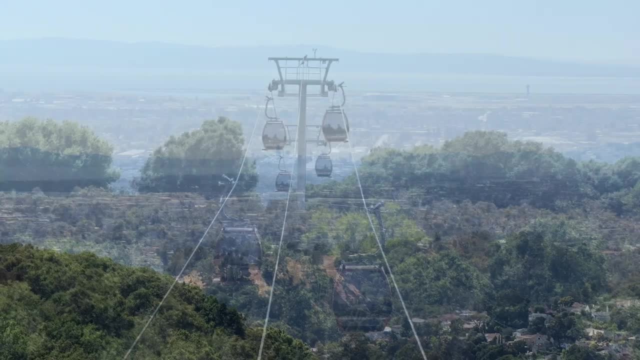 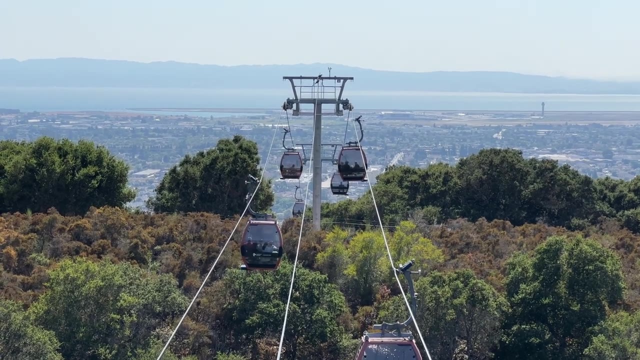 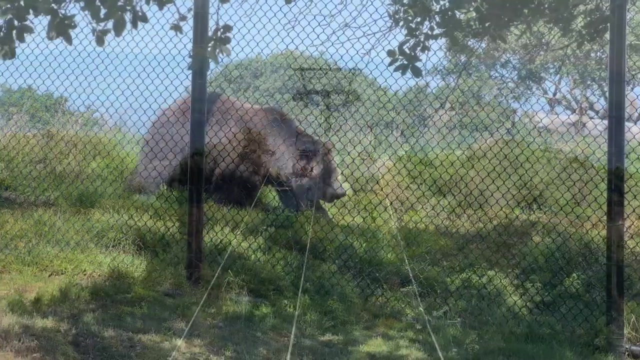 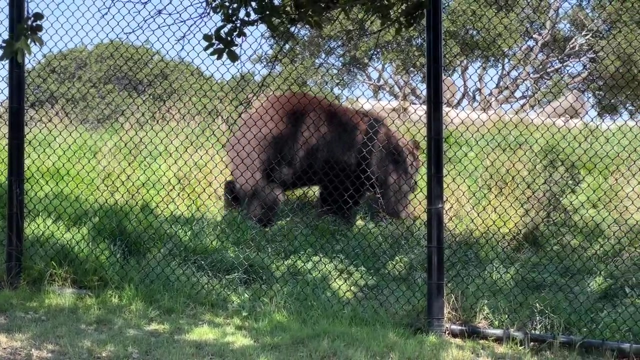 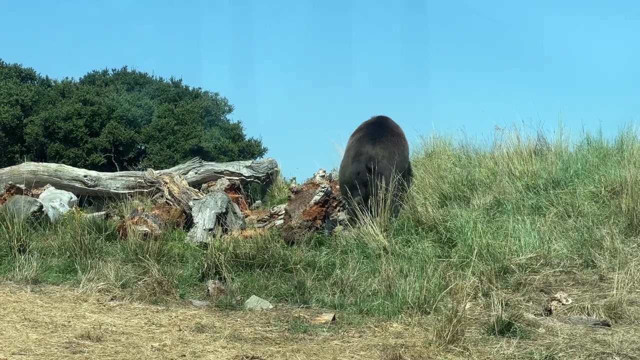 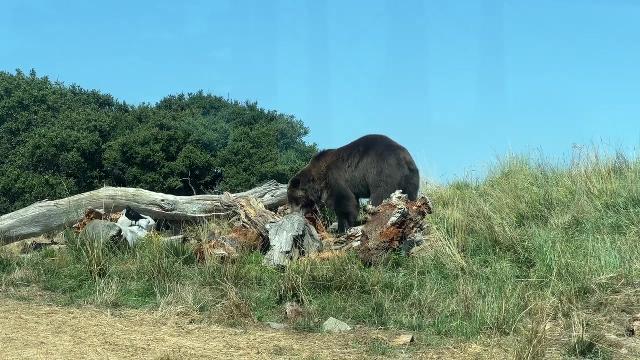 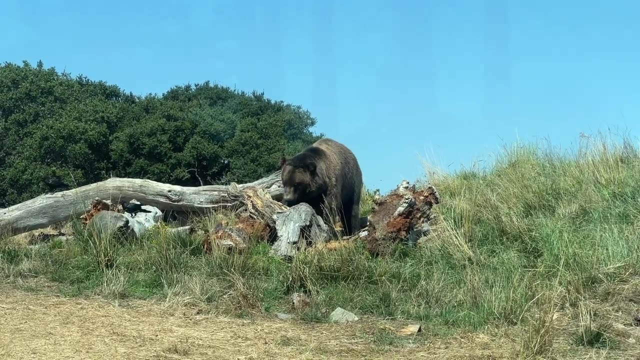 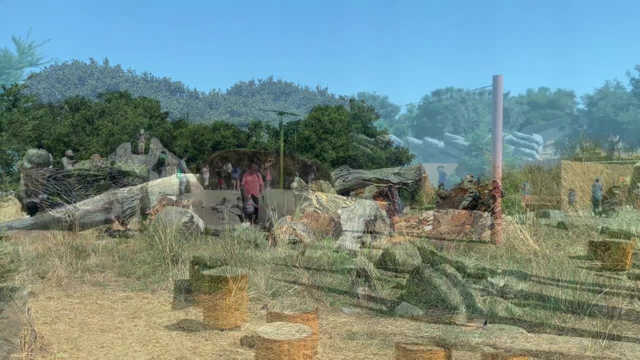 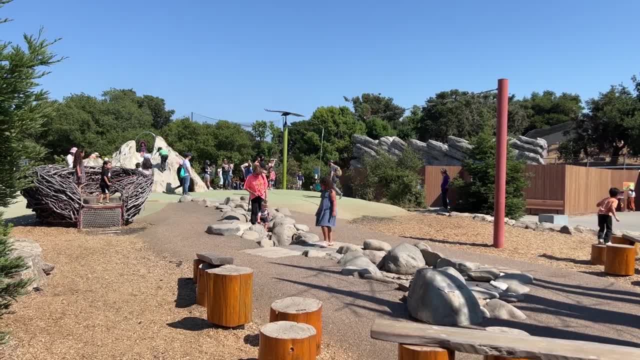 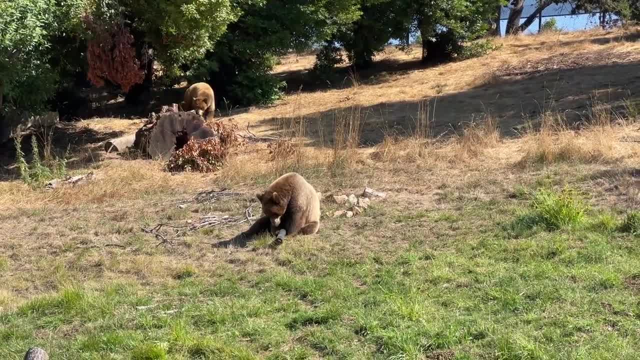 the California Trail region is popular with the displays of the grizzly bear, food and drinks, and we have look around helps. the kids also love this place because of the the playground and it offer plenty of games for children and Bye for now kids to play around. This is the black bear. It's much smaller and less. 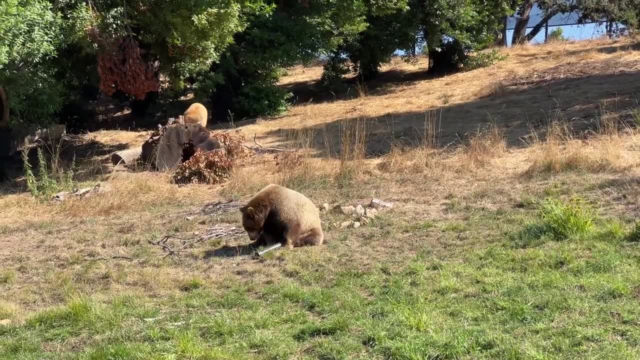 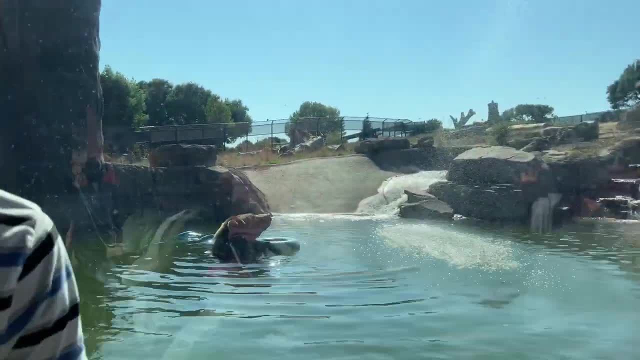 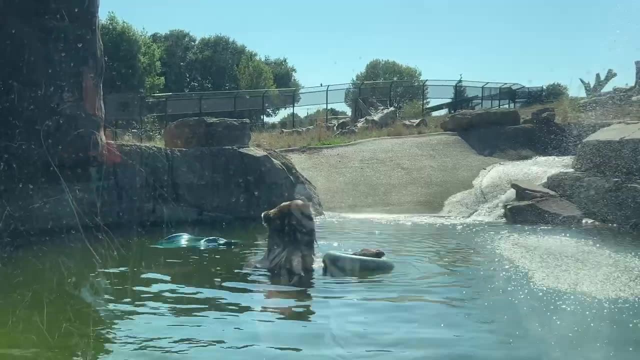 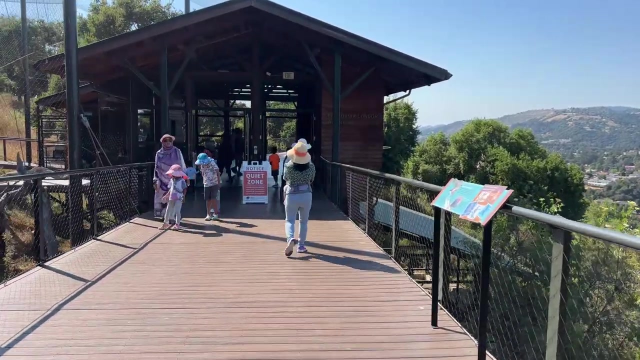 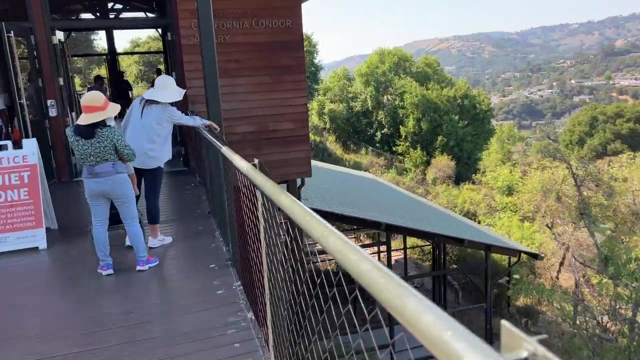 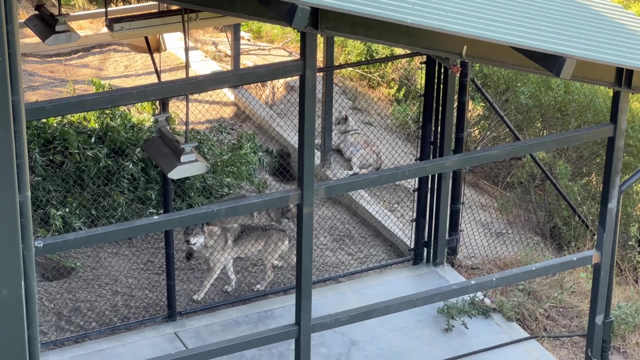 aggressive than the grizzly bear. We took the trail in the counterclockwise direction. Unfortunately, the mountain lion and the jaguar: they are sleeping, so not much to see about them. However, we can view all the animals, such as the gray wolf and, of course, the super. 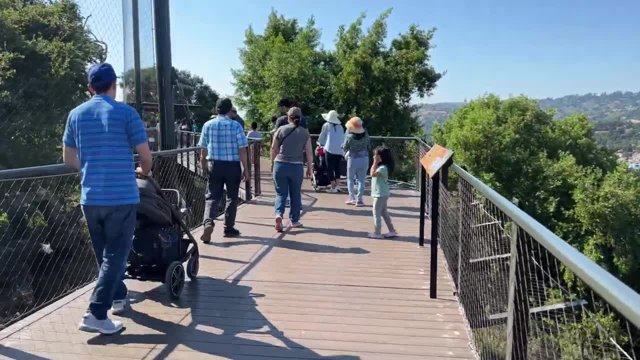 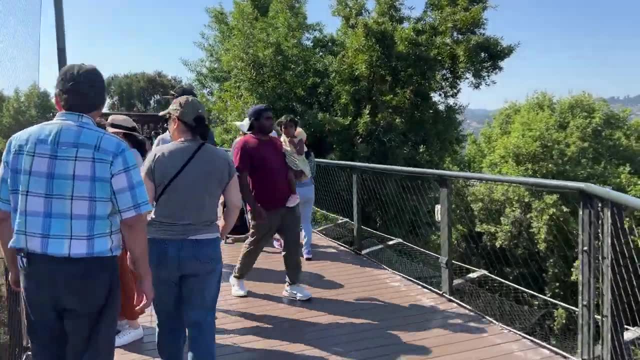 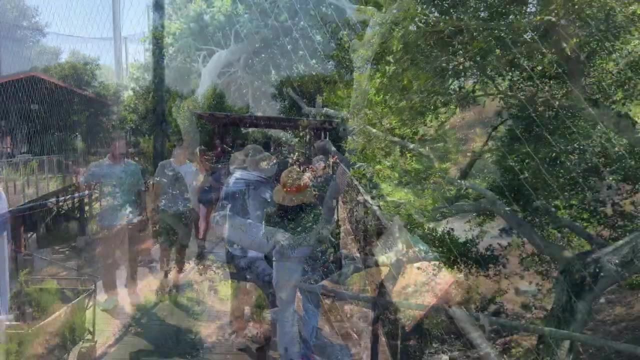 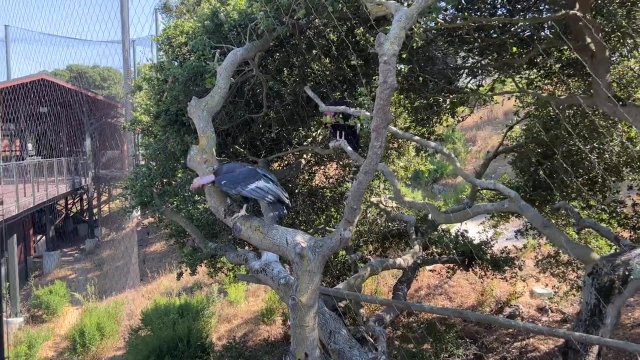 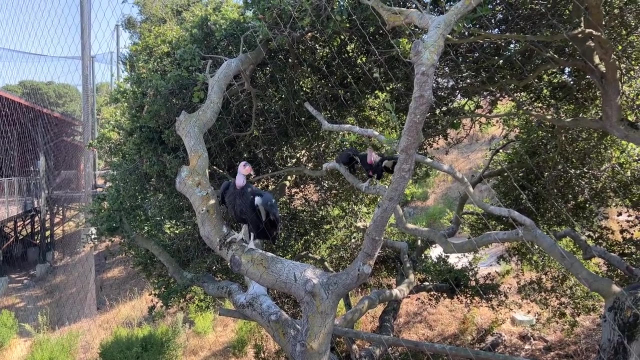 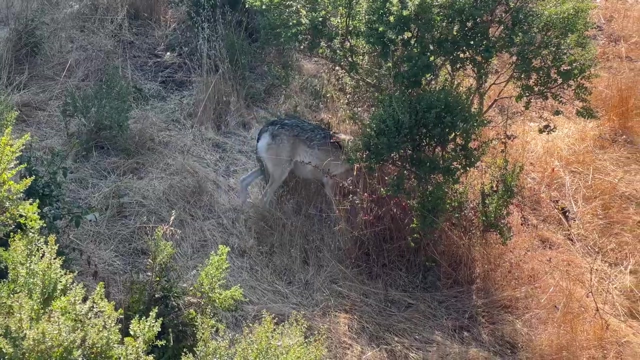 nice view of the Bay Area below. This is not a vulture but a California condo. It is big and it has a huge wind span of up to 14 feet or 4 meters. Wow, pretty nice view of the Bay Area. You can actually see it from the top of the mountain. 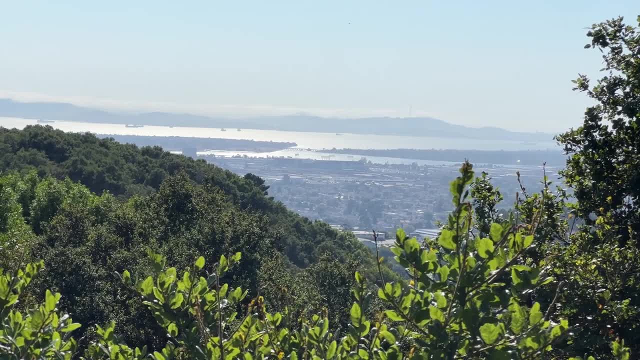 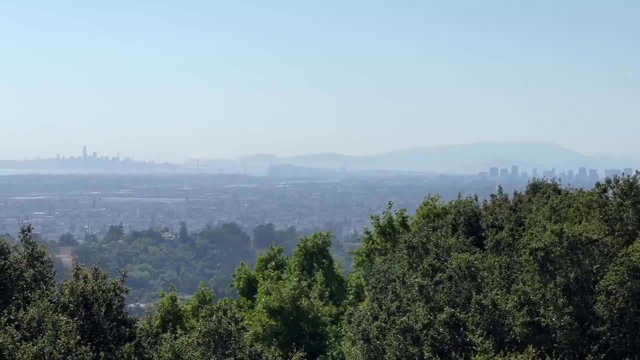 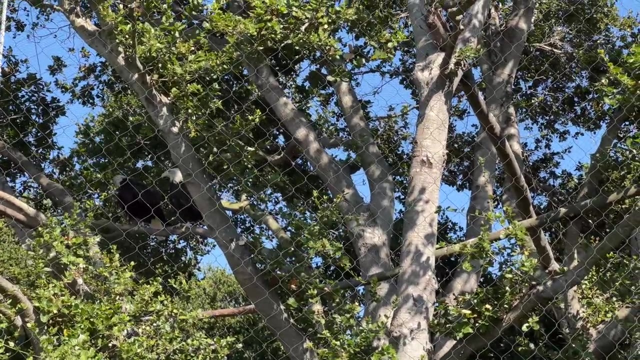 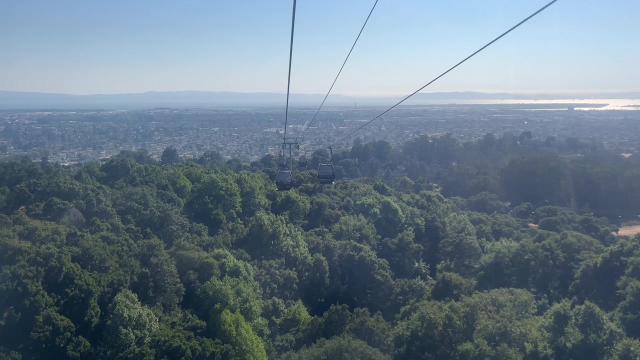 Wow, pretty nice view of the Bay Area. You can actually see it from the top of the mountain. We are in San Francisco and Delta Oakland. We take the gondola, ride down and get to the last area that we haven't been to. 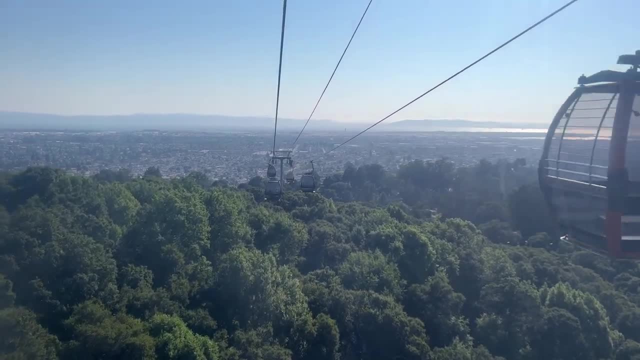 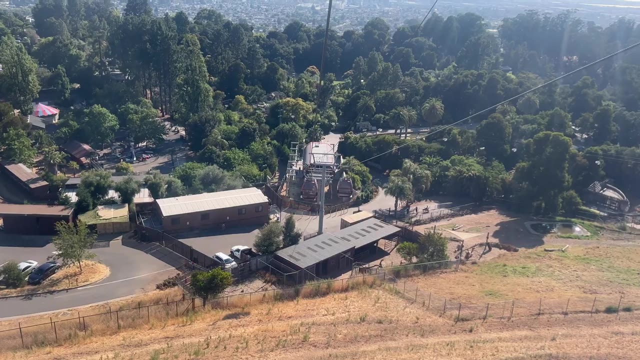 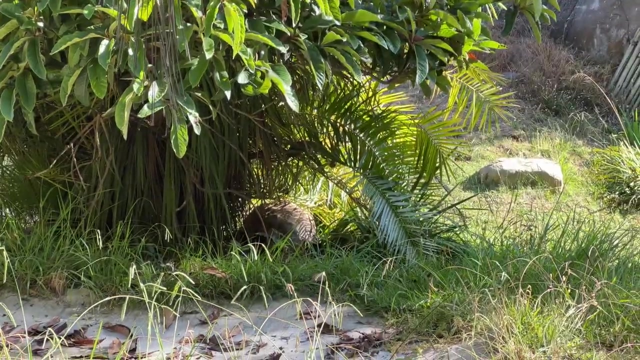 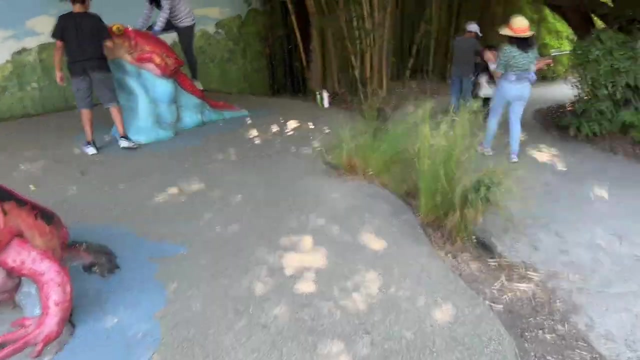 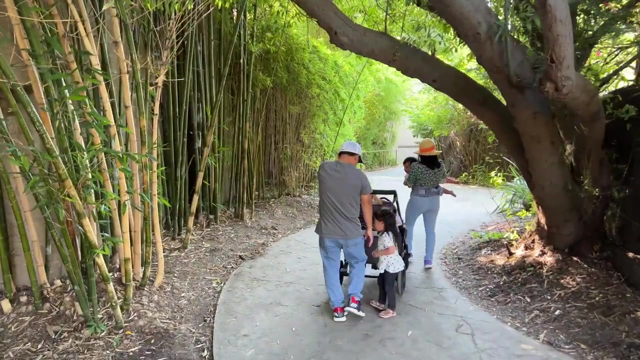 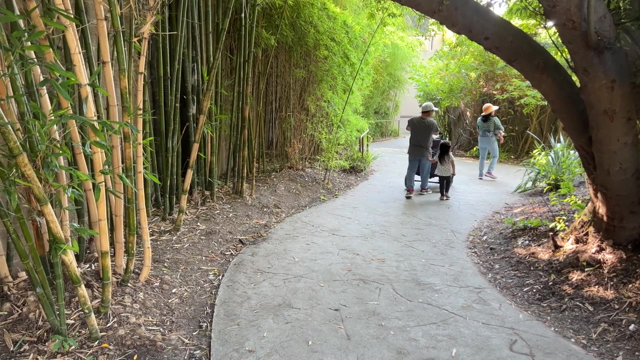 We just went to Wayne and Gladys Valley Children's Center. We just went to Wayne and Gladys Valley Children's Center, Valley Children Zoo to see tortoise, rabbit, house of bug, alligator, reptile and amphibian room. The reptile and amphibian room is pretty nice. It features frogs of. 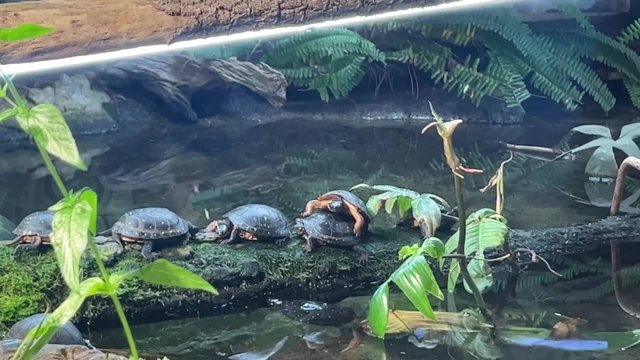 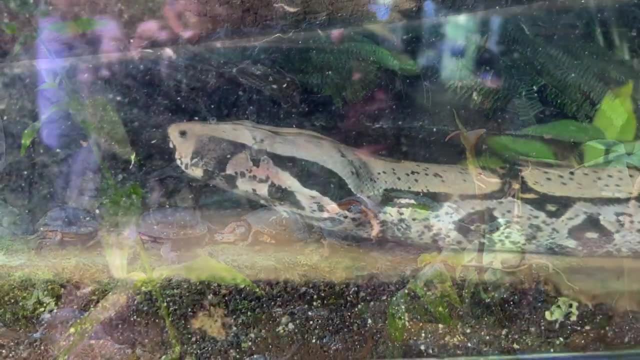 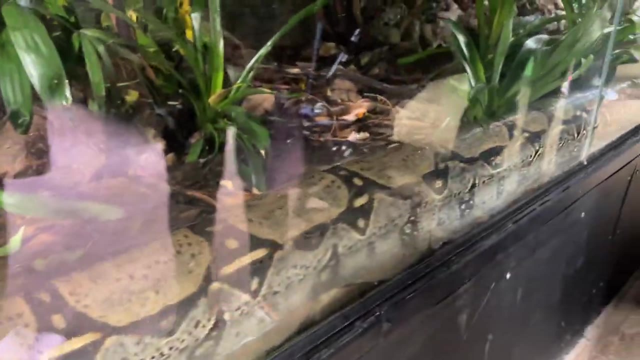 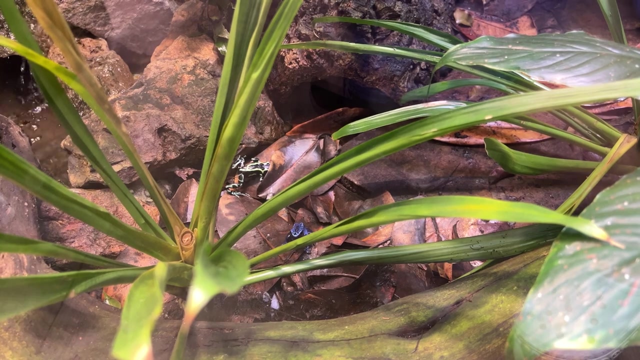 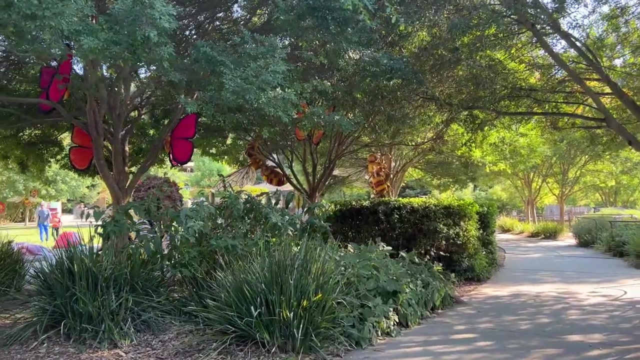 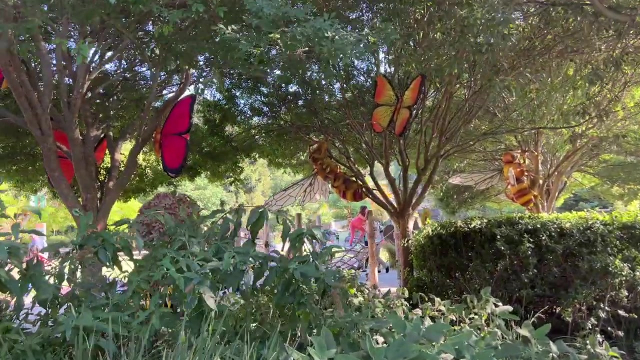 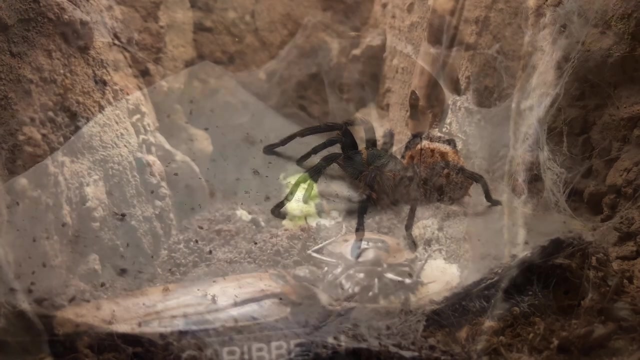 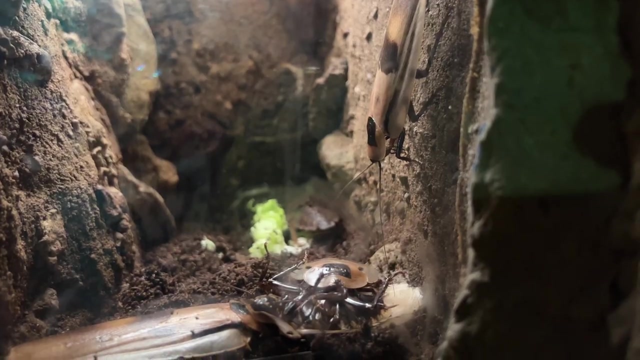 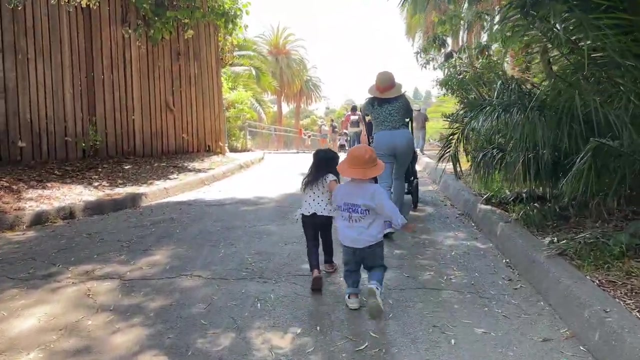 different color and turtles mating with each other. haha, The alligator is sleeping and we can't even see it. so we get to the house of bug to see some spider cockroaches. we went to the zoo from 10: 30 to 5: 30, pretty exhausted after all the walk.